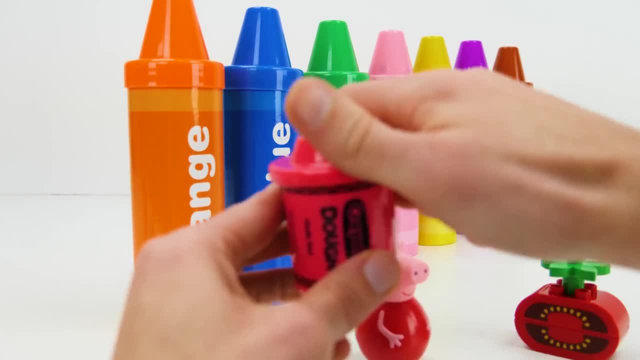 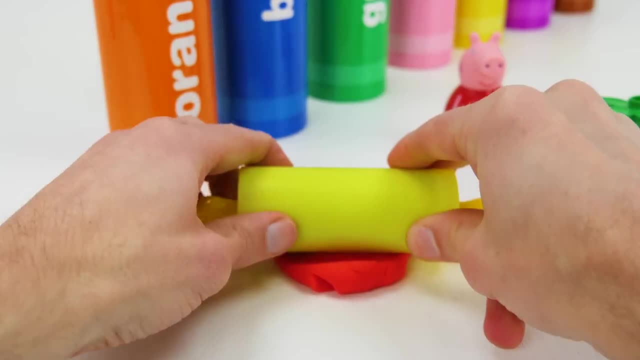 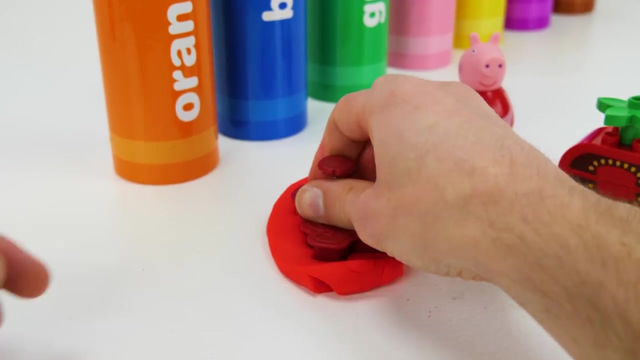 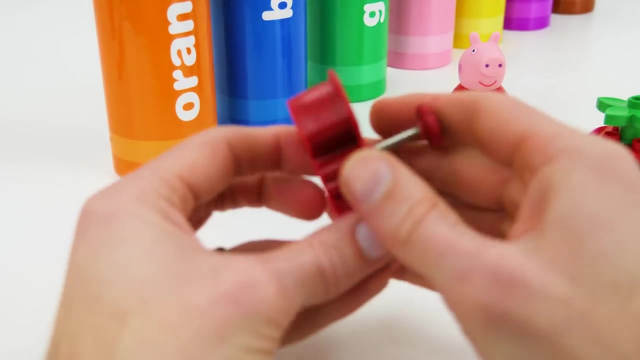 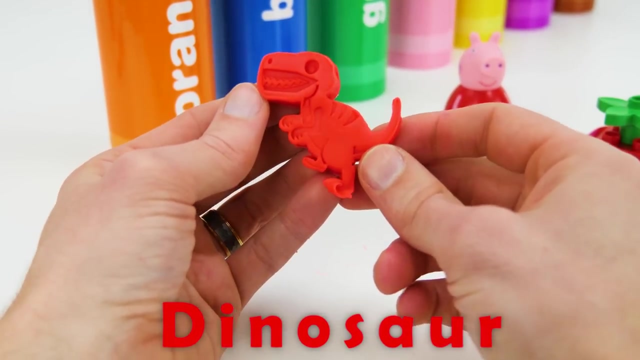 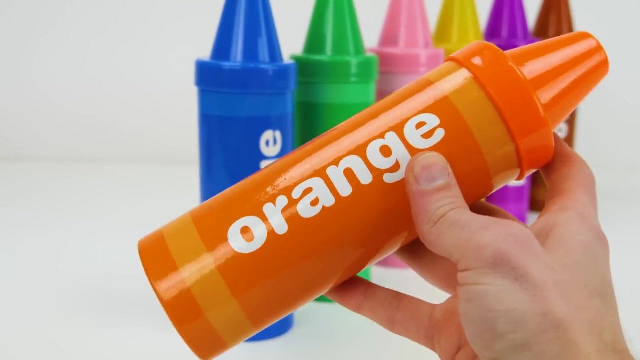 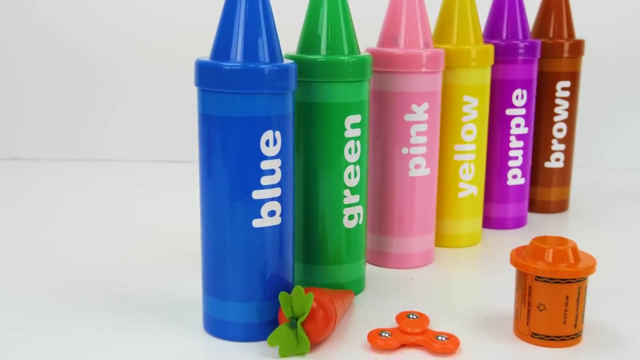 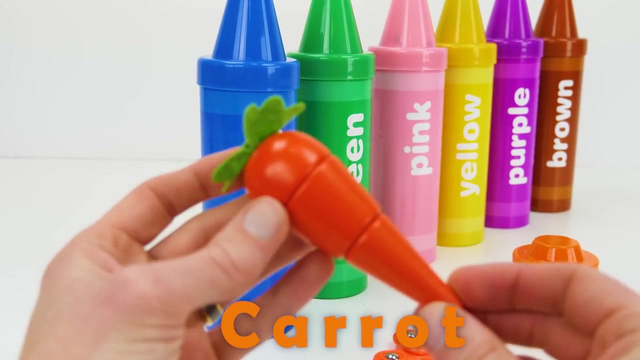 Red Play-Doh, Let's roll it out to be flat Red Cutter Dinosaur. Now for our second color: orange Spinner, Spinner. The spinner is spinning Carrot. A carrot is good for you. We can cut it into two, three pieces. 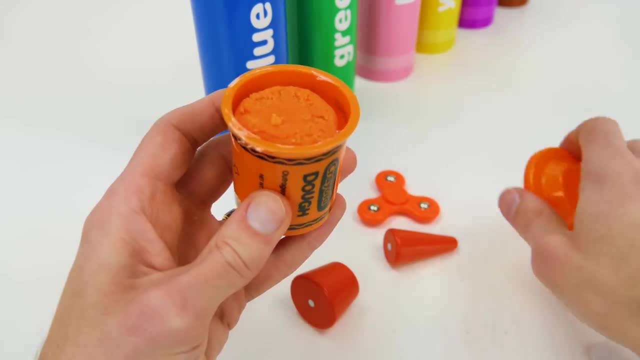 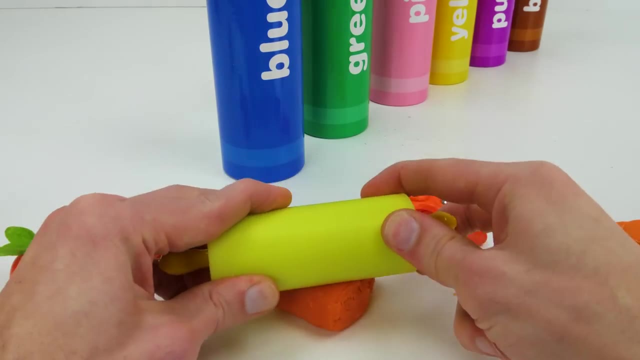 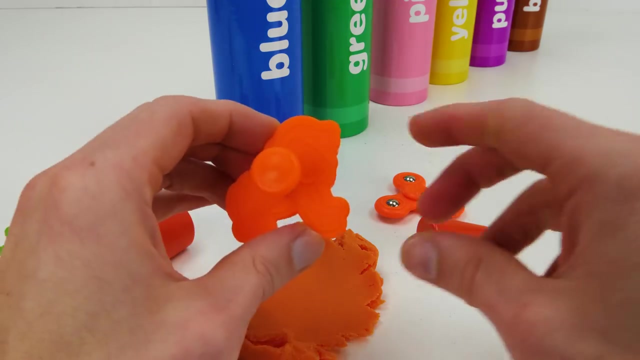 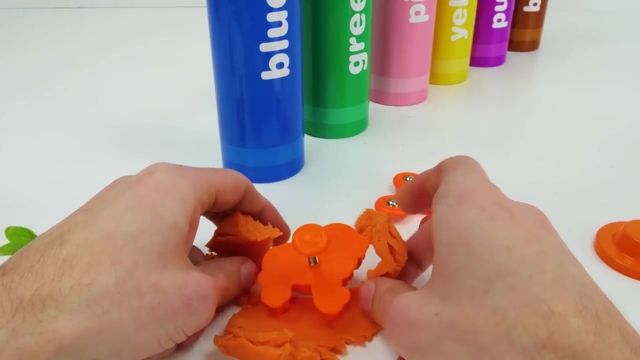 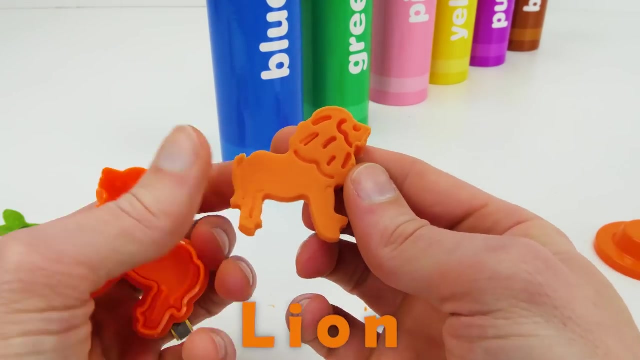 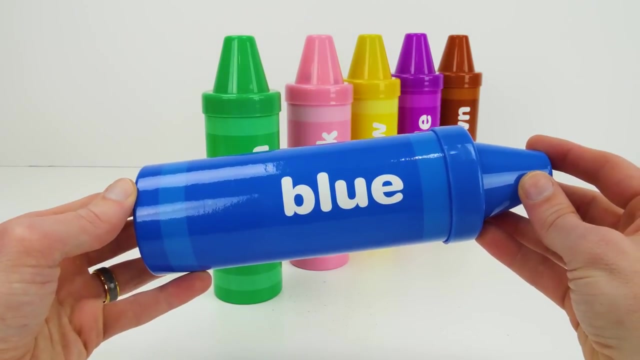 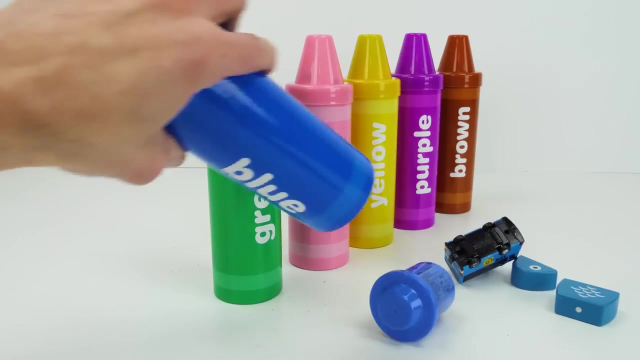 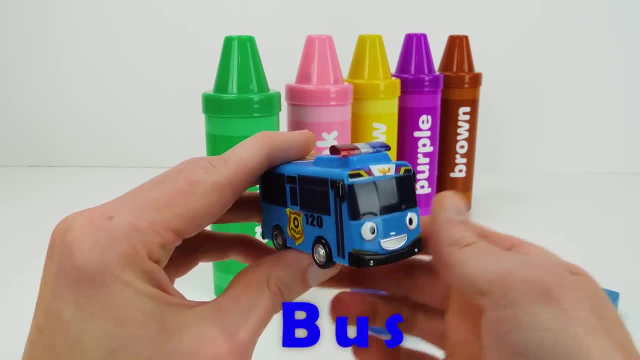 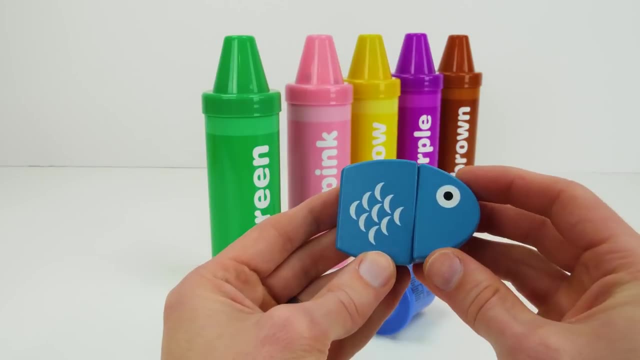 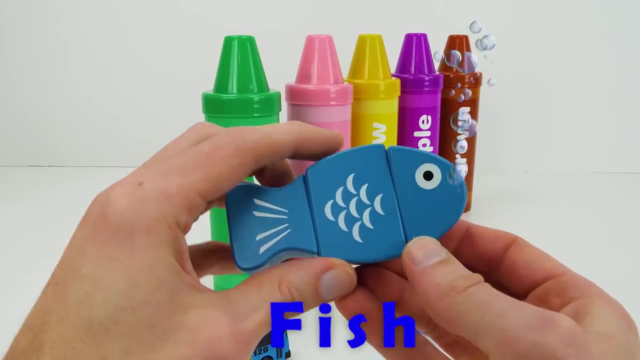 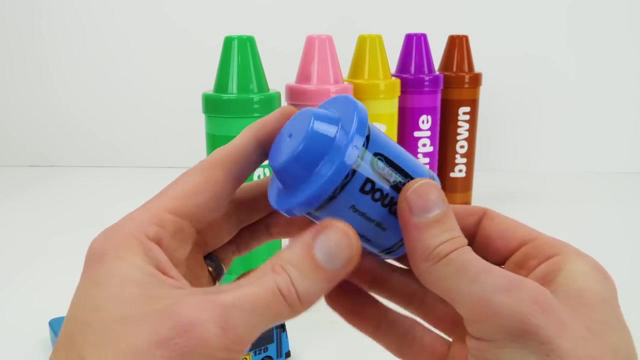 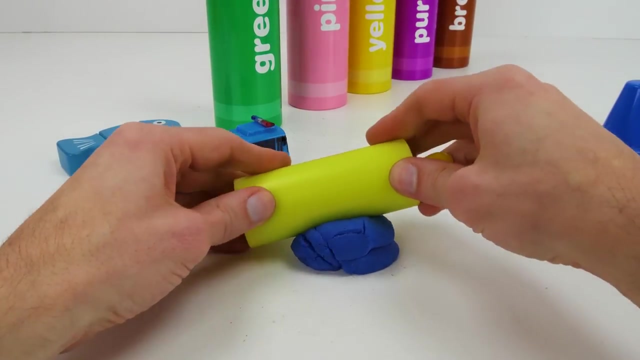 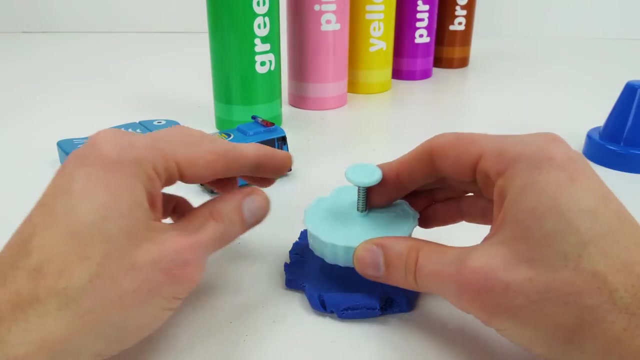 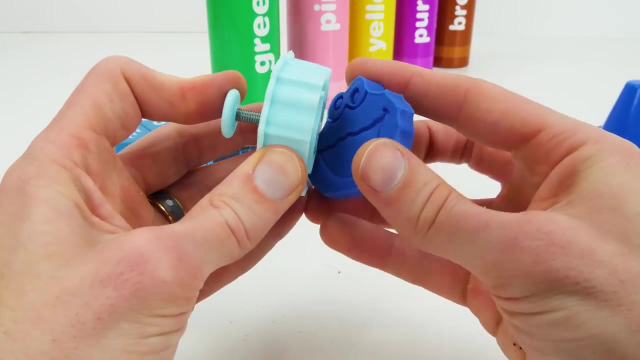 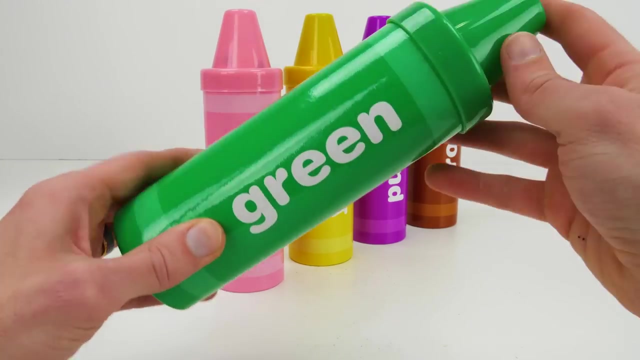 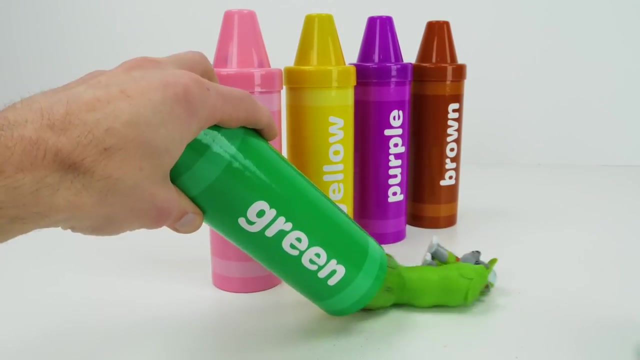 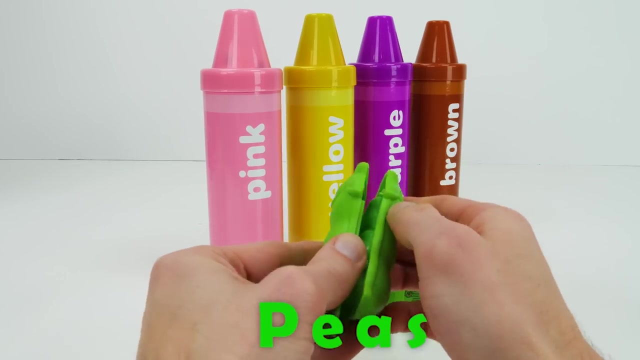 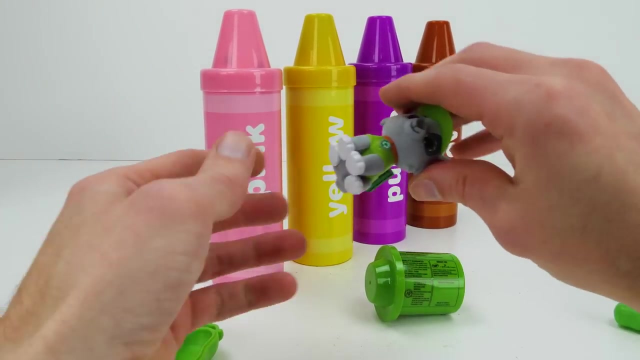 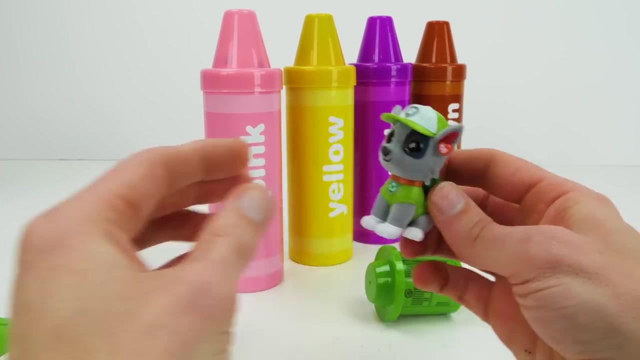 The bus has a siren. Fish Fish live in water. Fish Fish live in water. Fish Fish live in water. blue play-doh, blue cutter cookie monster. our fourth crayon is green peas. peas coming up high, rocky, rocky is from paw patrol. green means go. 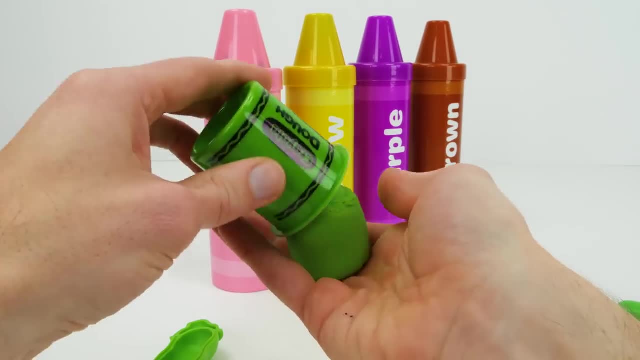 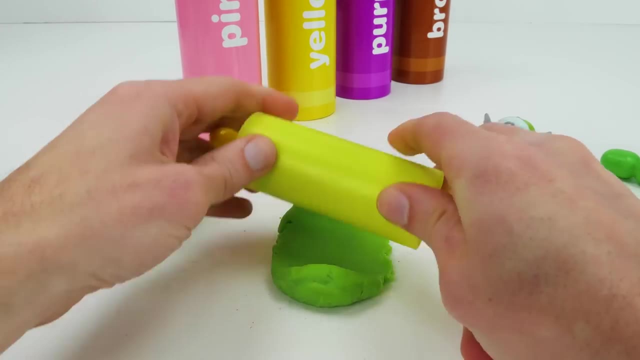 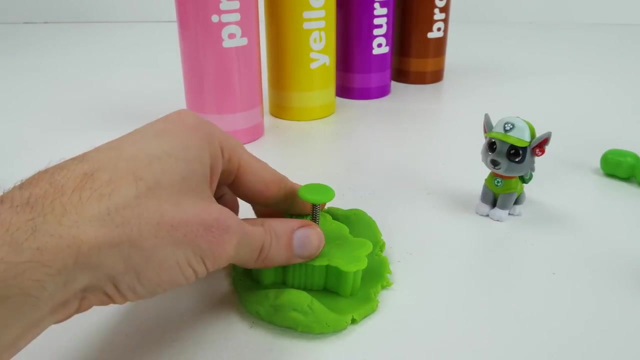 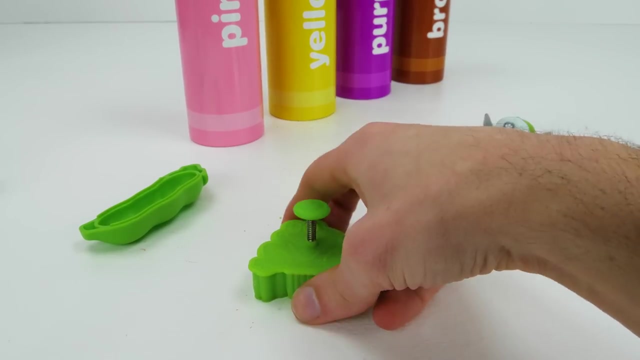 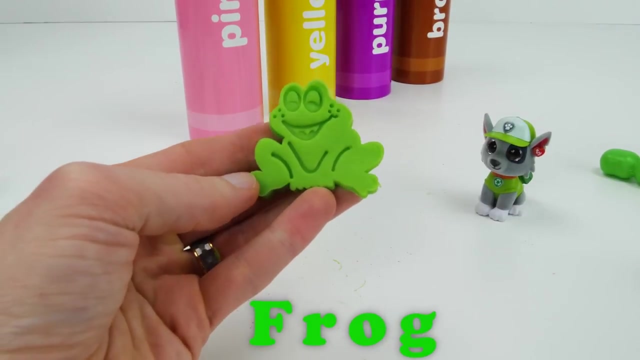 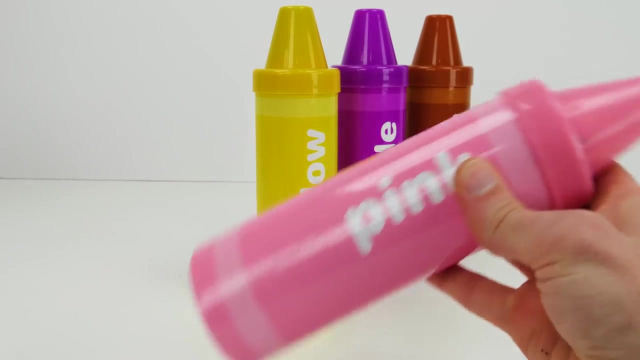 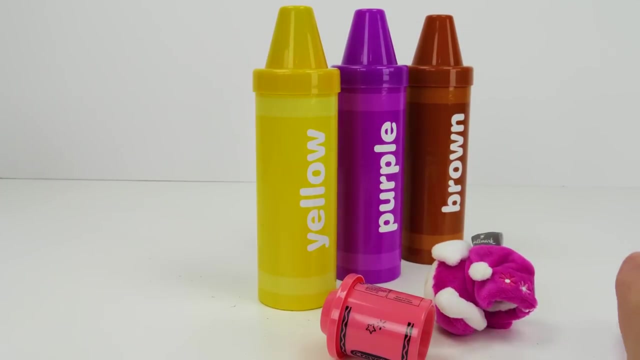 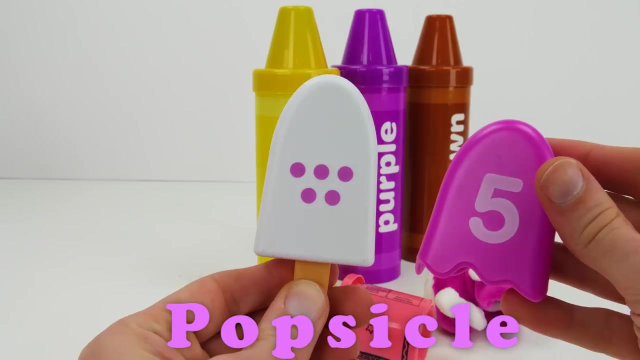 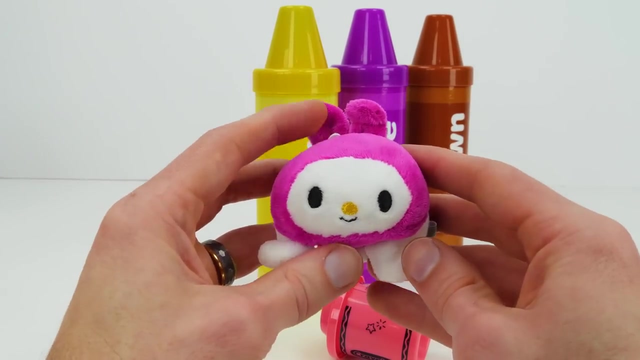 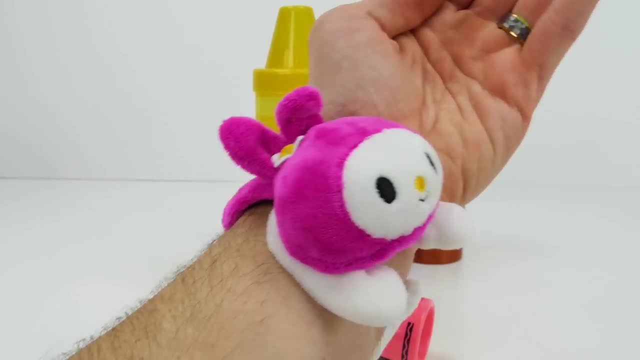 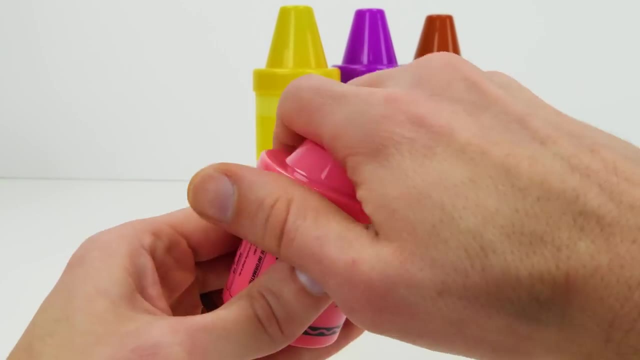 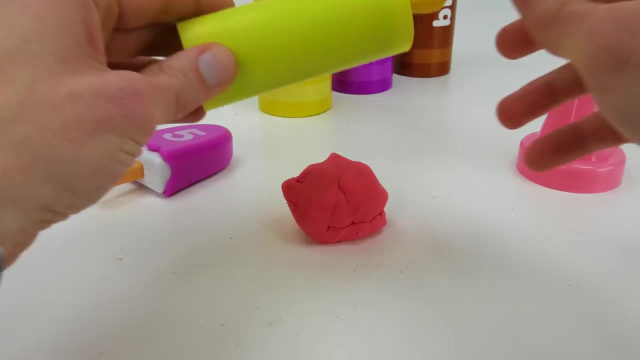 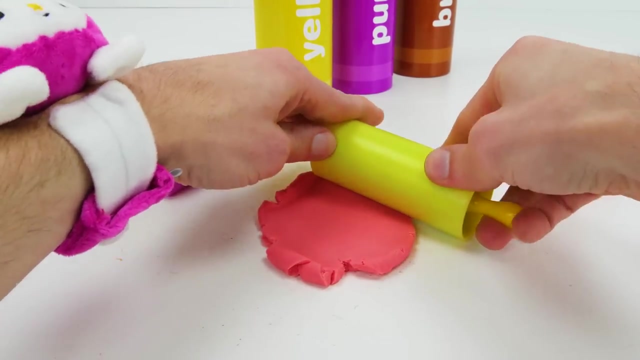 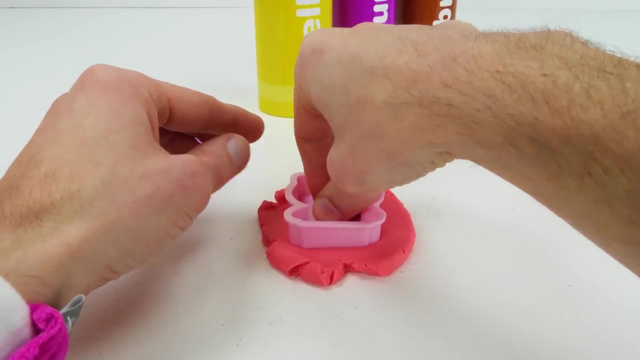 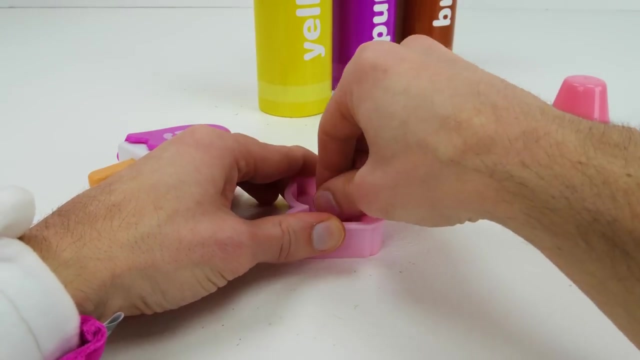 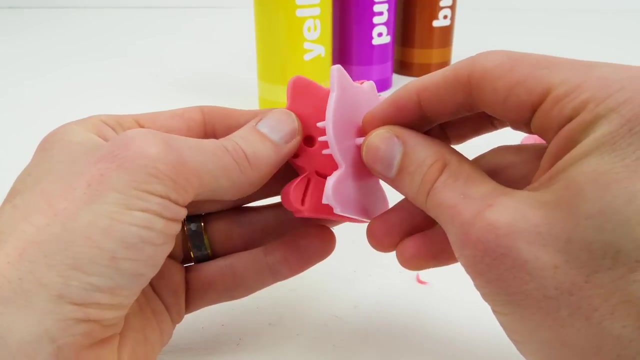 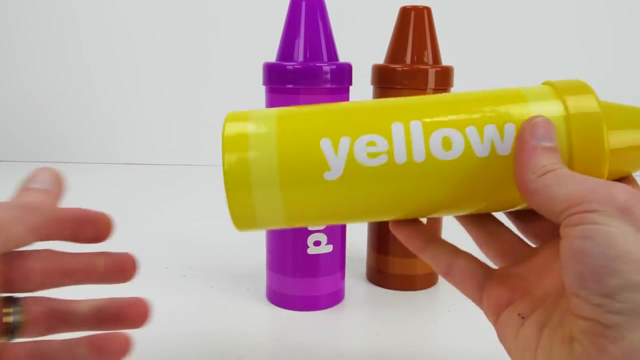 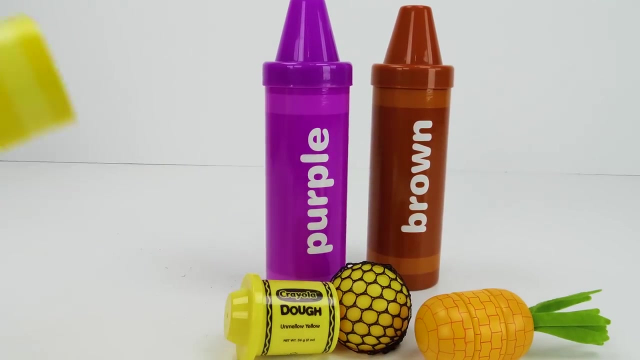 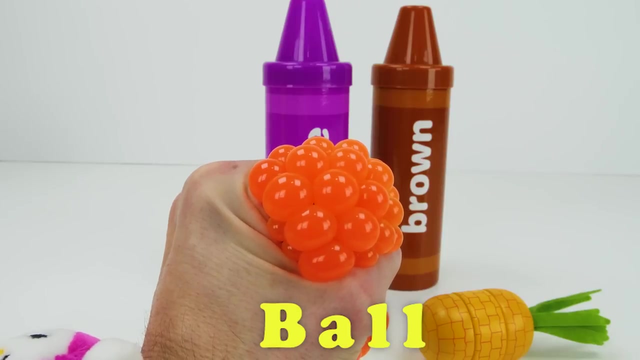 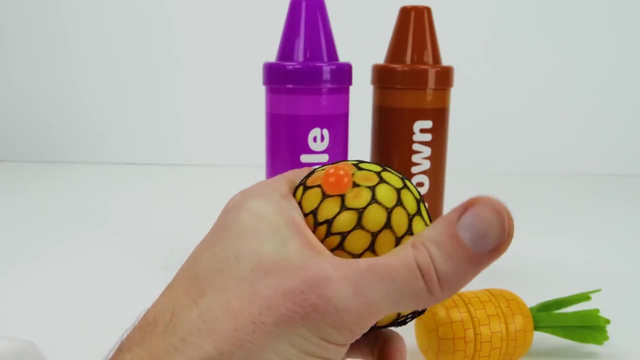 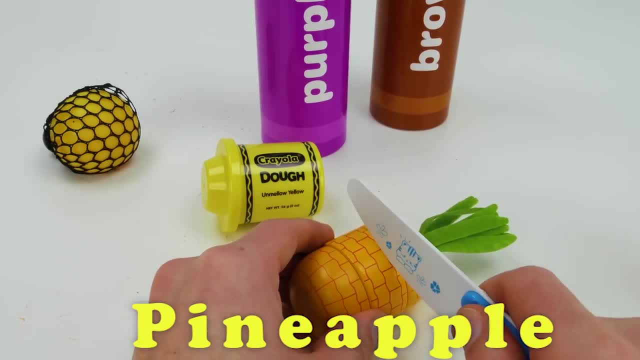 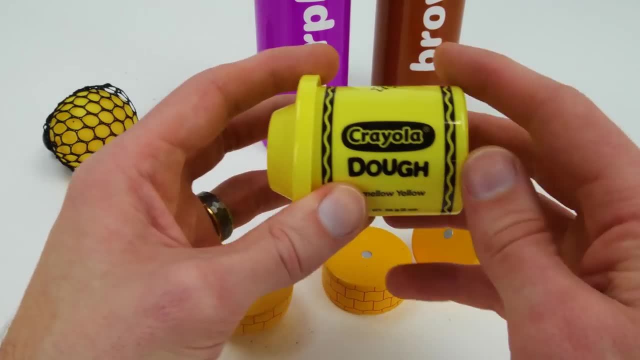 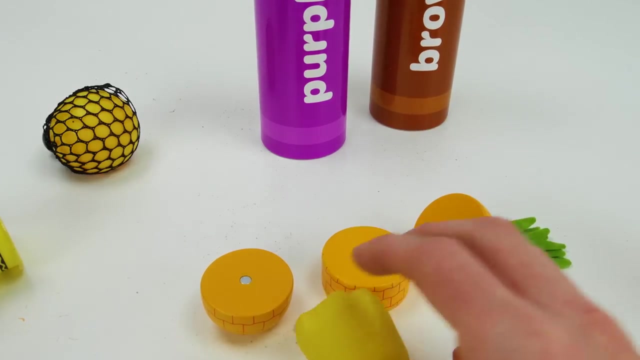 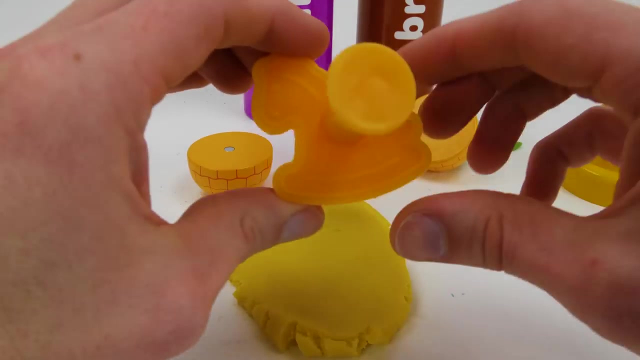 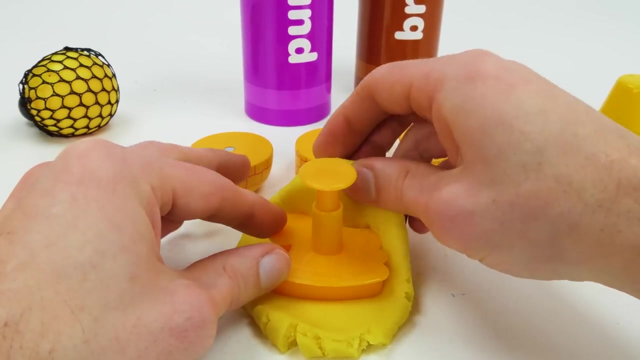 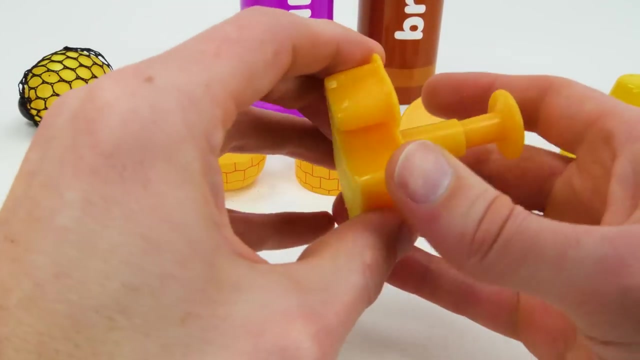 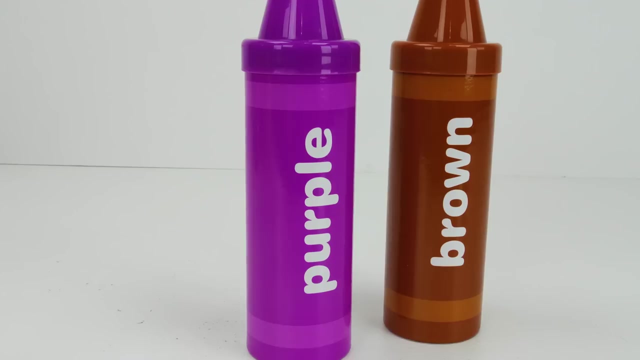 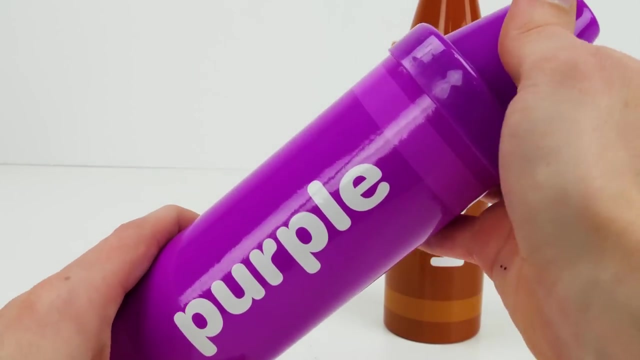 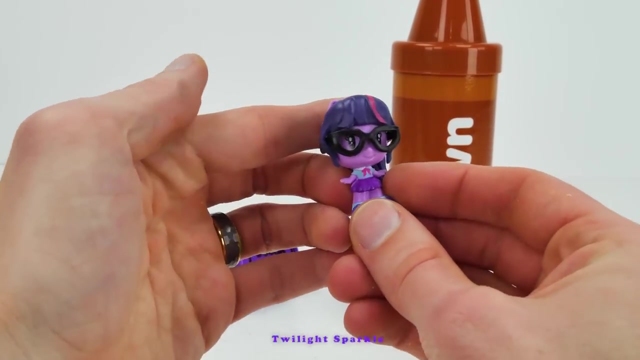 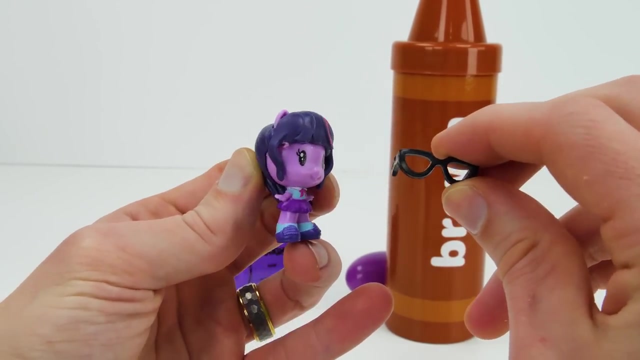 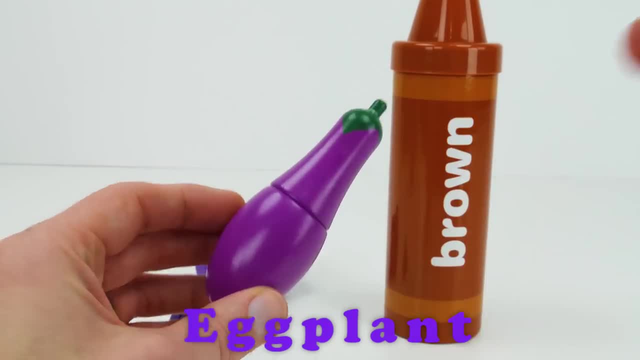 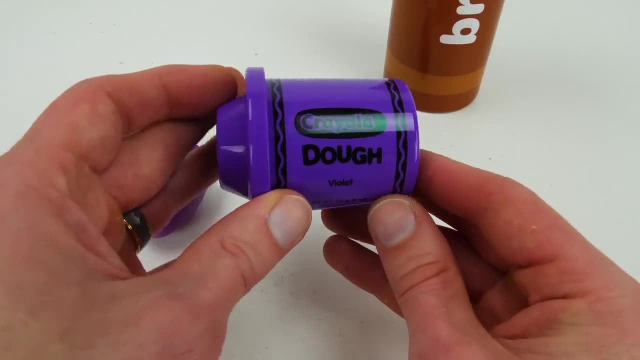 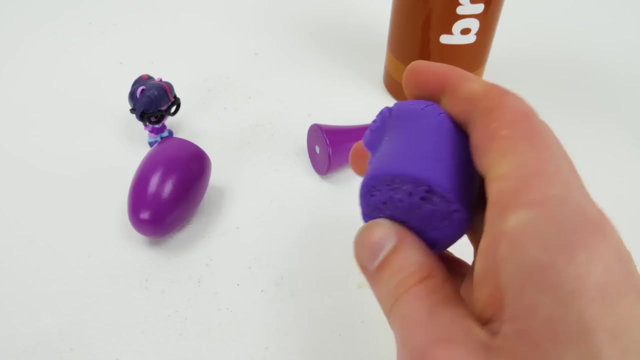 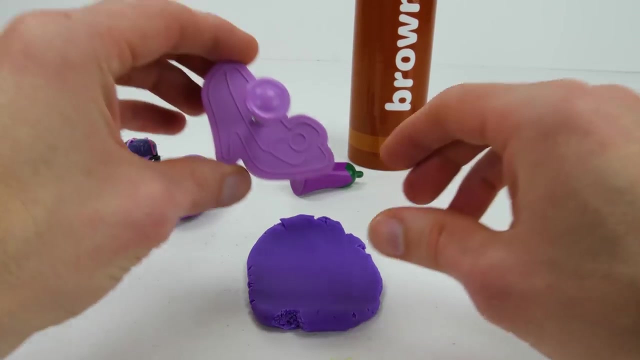 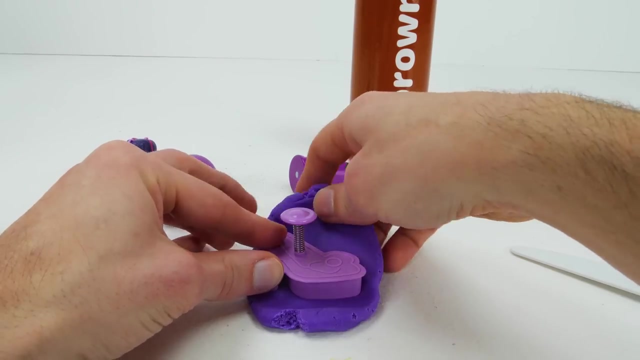 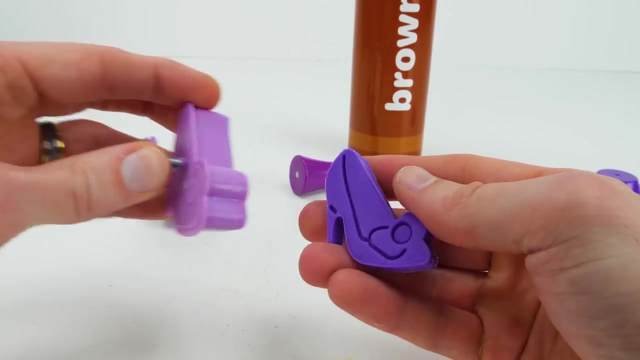 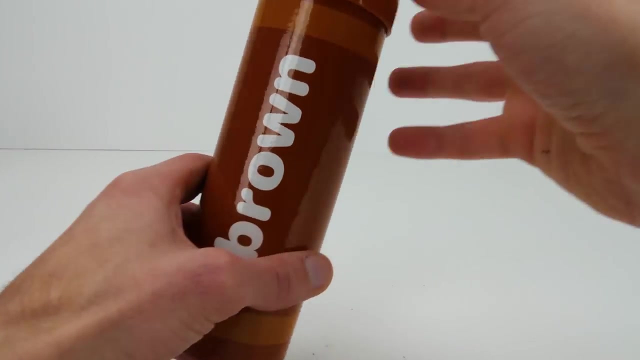 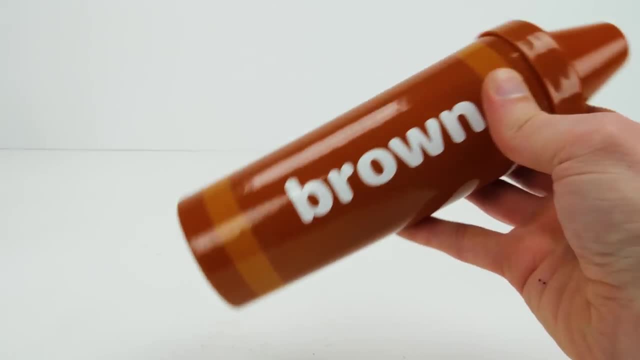 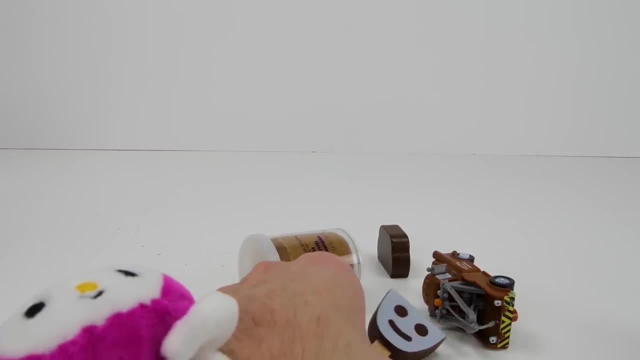 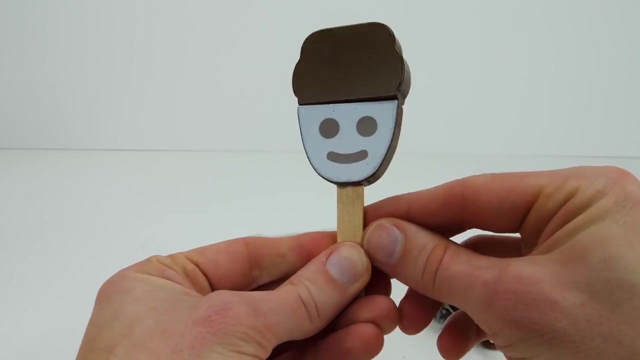 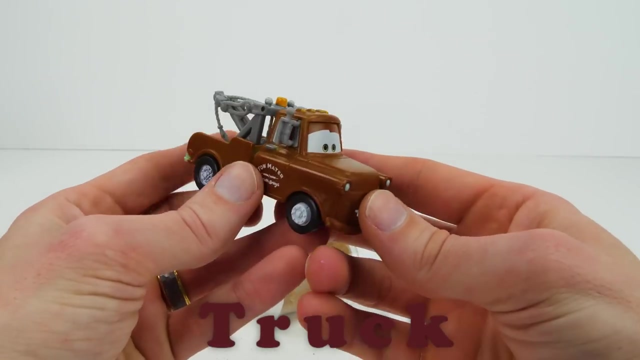 She really likes to play with food and dumplings, Even if it only has one school And this is the only one, she has Charcoal Brown Ice Cream. This ice cream comes in black- has a smiley face truck. this truck is named mater. watch this with some warm. 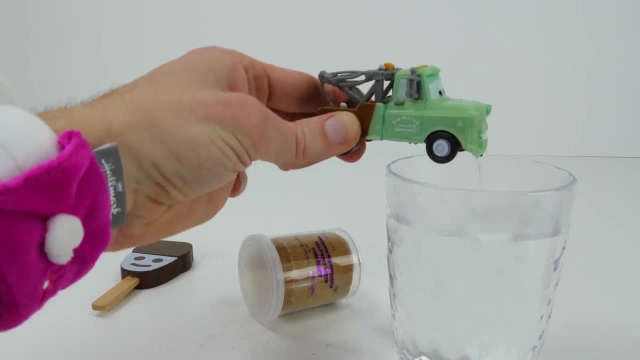 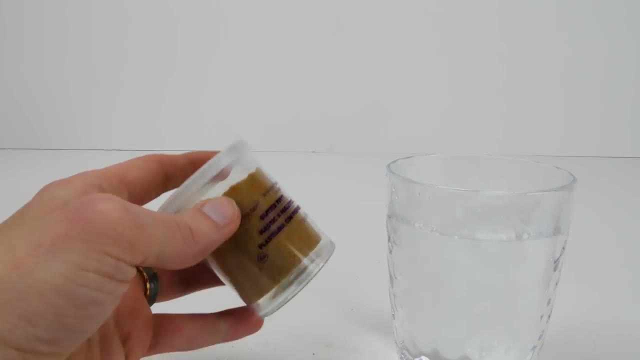 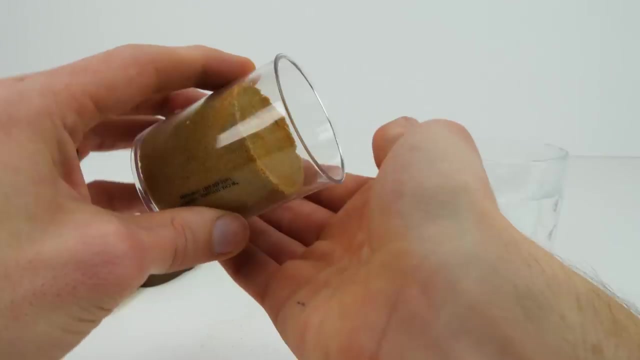 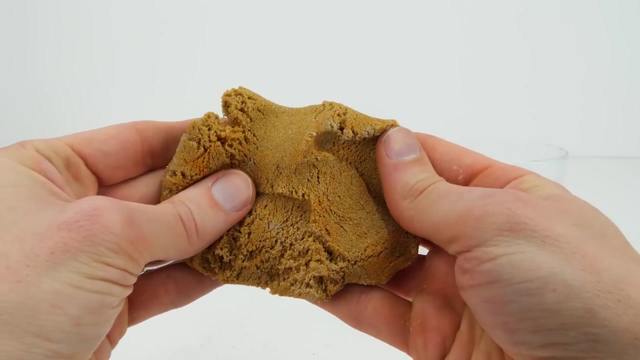 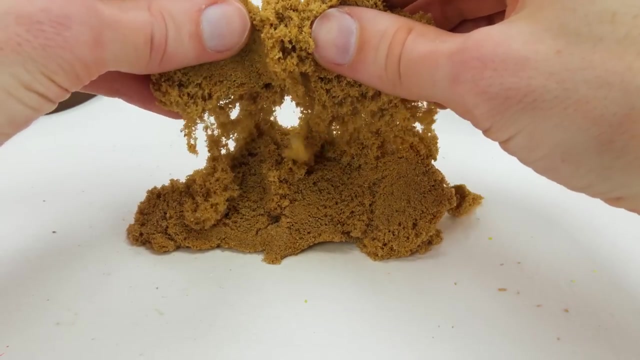 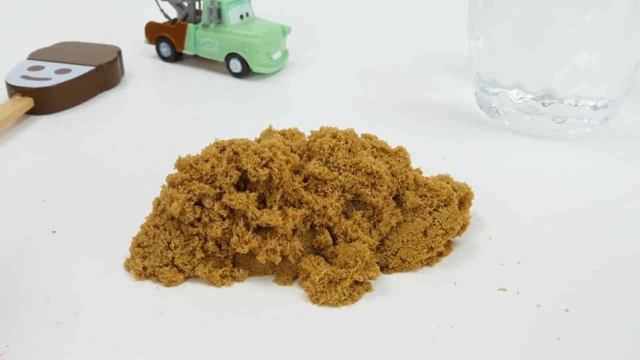 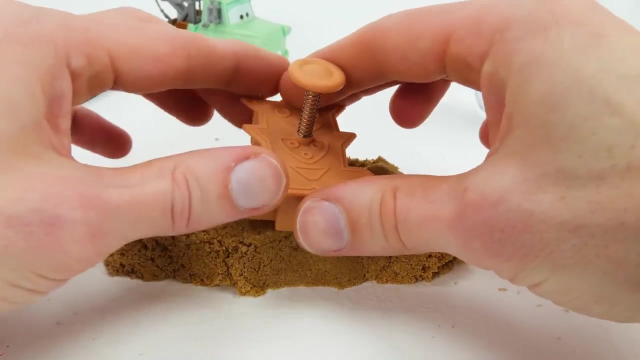 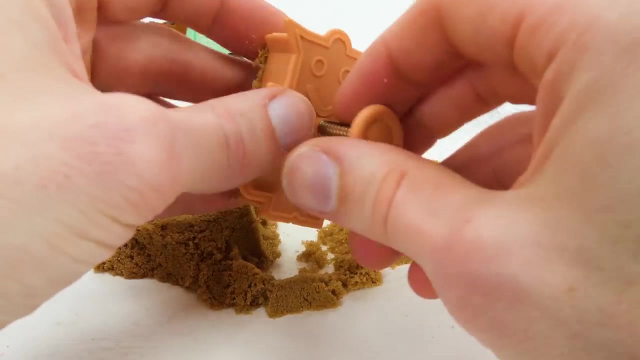 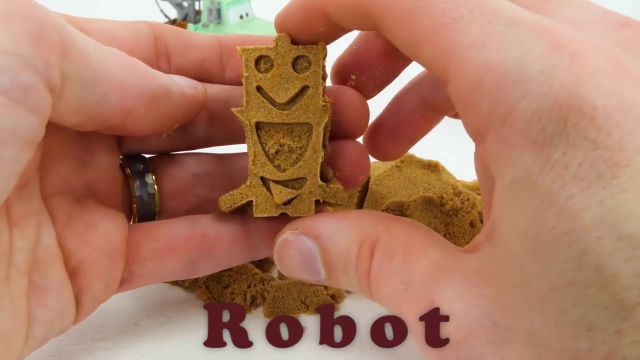 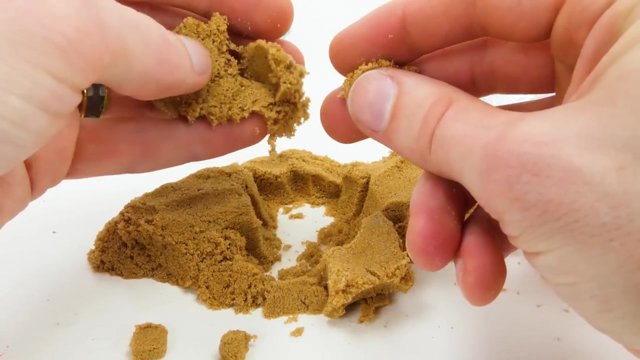 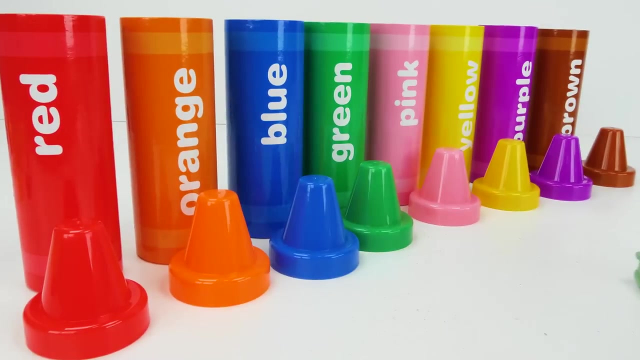 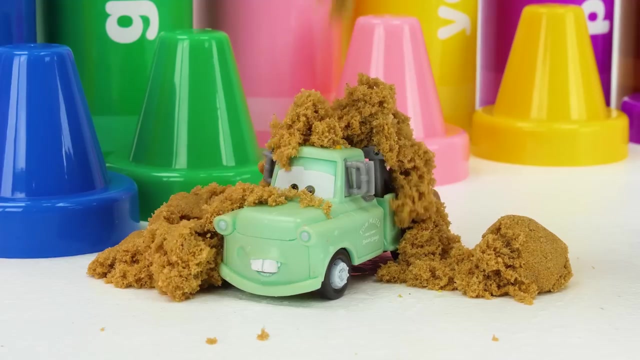 water we can change mater to green brown kinetic sand. it feels neato brown cutter robot there. now we've played with all of our colors. bye guys. if you like the video, give it a thumbs up. that was fun. hey, what's the big idea? oh no, hey, there's sand in my radiator.